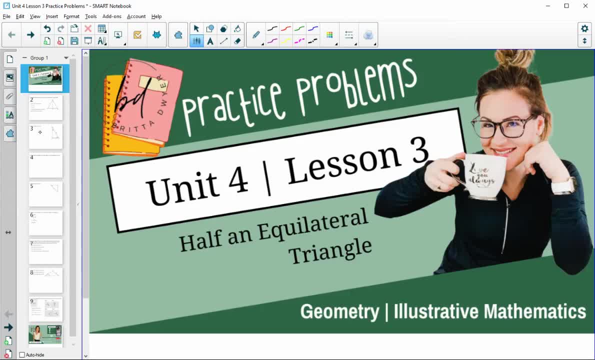 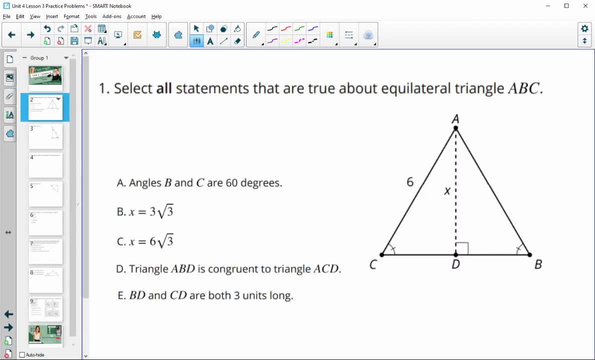 In this video we're going to take a look at the Unit 4, Lesson 3 practice problems. So number one asks us to select all true statements about this equilateral triangle, First statement being that angle B and angle C are 60 degrees. We know that that's true because 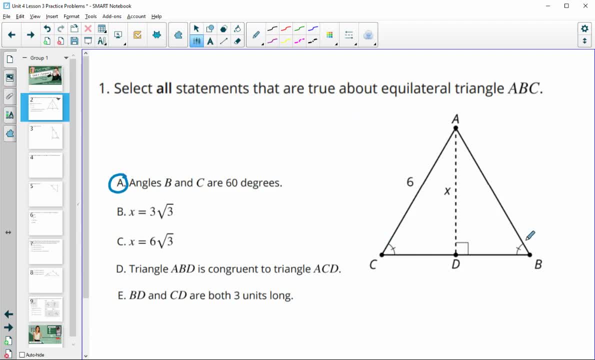 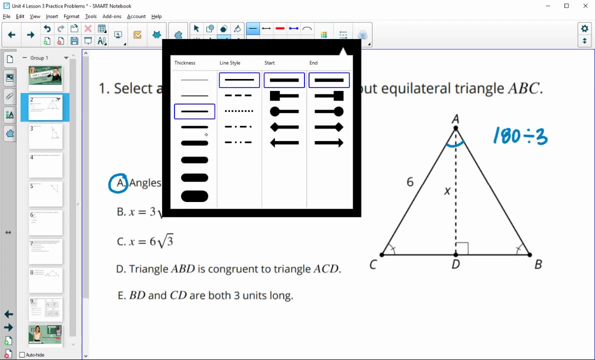 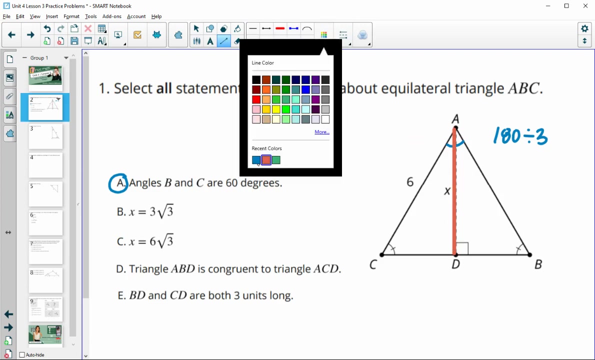 an equilateral triangle is also equiangular, So B and C are equal and so is this larger angle A. So if we do 180 divided by 3, we get 60 for each of those angles. B asks us if this altitude here is 3, square root 3.. So this altitude here is actually taking this. 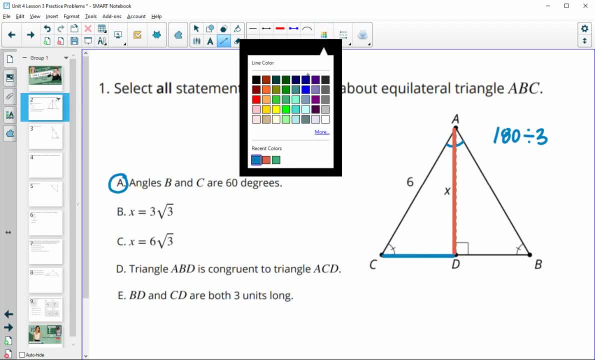 little short leg here times the square root of 3.. And we know that this little short leg here is half that Hypotenuse, So this leg here is 3.. And then we take the blue segment: times the square root of 3. 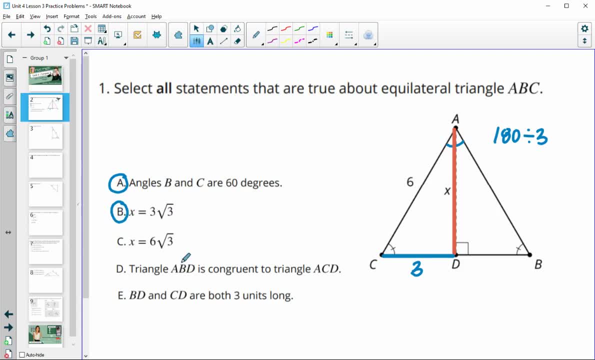 to get this orange one. So we do know that it's 3 square root 3.. So then it would not be 6 square root 3.. And then triangle ABD. So ABD, this one on the right, is congruent to ACD. We know that. 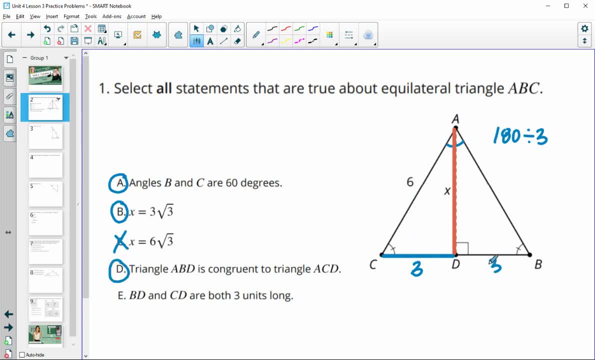 that is true because we also know that this one is 3. They share this 9. There's lots of different ways you can prove that these are congruent. We know it's equilateral, So this is 6. We know they share this side. So you could do by side side side. You could do by. 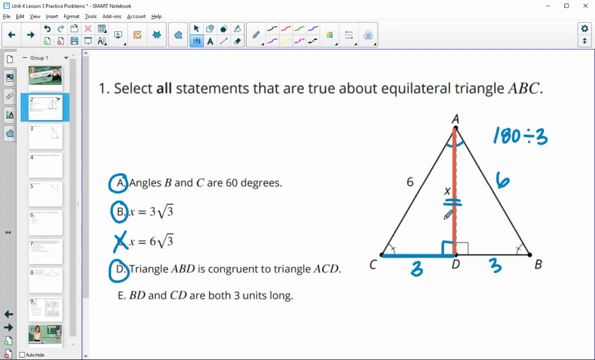 side, angle side, You could say by angle side, angle. Lots of ways to prove that those two triangles are congruent. And then BD and CD are both 3 units long. That's true because it cuts this 6 in half. 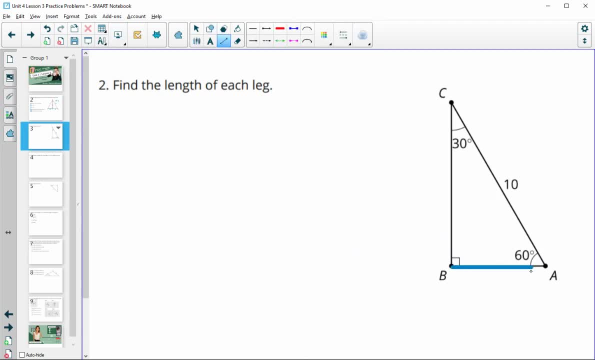 Number 2, find the length of each leg. So we know that this one is always half of the hypotenuse. And then we know that this one is the square root of 3 times longer than the blue one. So the blue one is 10 divided by 2, which is 5.. And then the orange one. 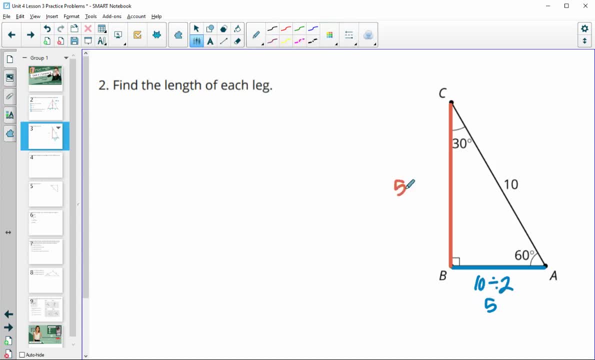 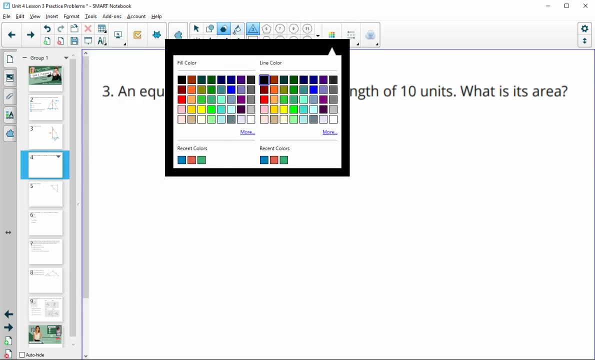 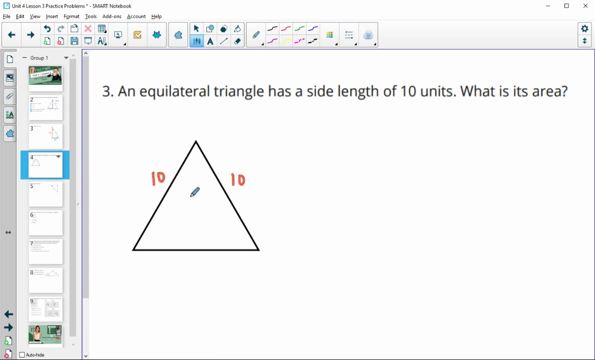 is the blue one times the square root of 3.. So 5 square root of 3.. Number 3,, an equilateral triangle, has side lengths of 10.. What is its area? So let's get a triangle drawn here And each of the sides is 10.. And then we want to know the area. So I'm going to leave. 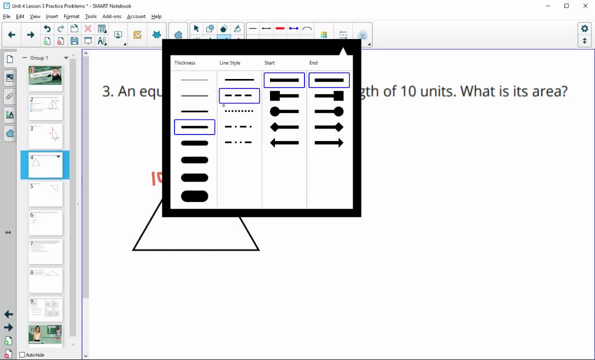 that bottom one blank, because in order to do the area, we need the height. So we're going to need to find this altitude, And to do that then we'll also take a look at how long this side is. So we know this little piece. 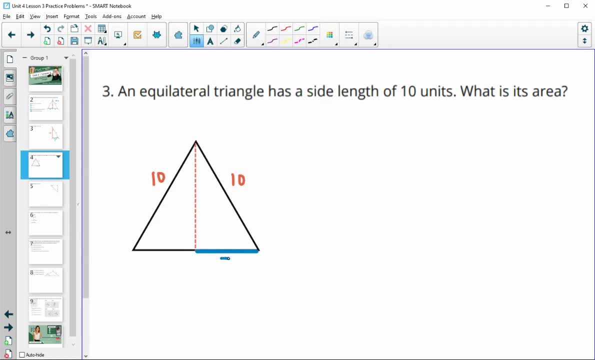 here is 5.. So it's half the full length And then that makes this altitude here 5 times the square root of 3.. So when we go to do the area of the triangle, we want to do the base times the height. 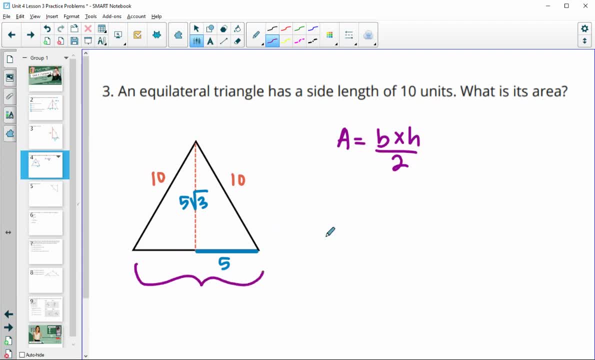 divided by 2.. The base here is going to be this whole thing, which is 10 times the height, Which is the altitude, or the 5 square root 3.. And then we want to divide by 2.. So 10 times 5 is. 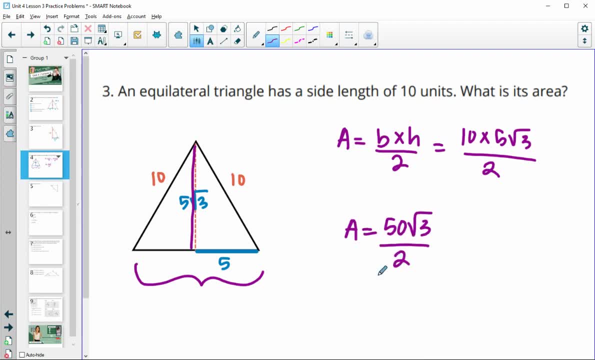 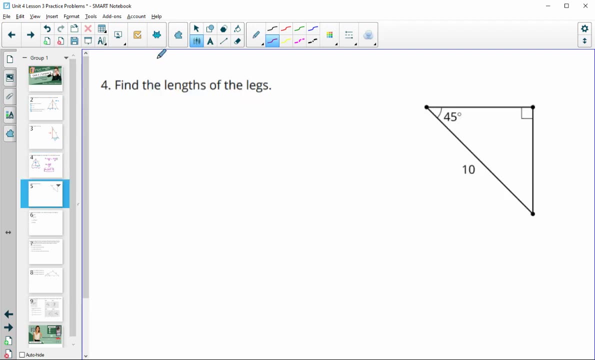 50 square root 3 for the top divided by 2.. 50 divided by 2 is 25.. So 25 square root 3 units squared would be our area Number 4, find the lengths of the legs. So now this one is back. 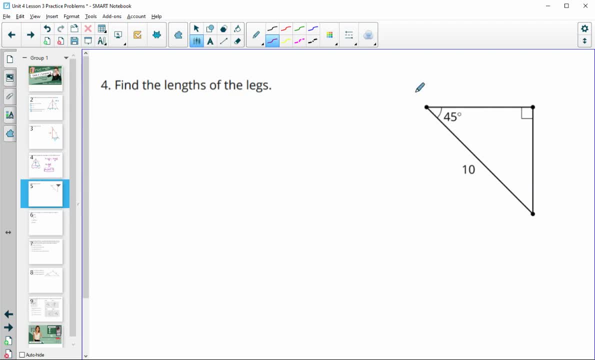 to a 45-45-90.. So this one's half of a square And if we remember the connection between the hypotenuse and the leg in a 45-45-90, they are multiplied or divided by the square root of 2.. 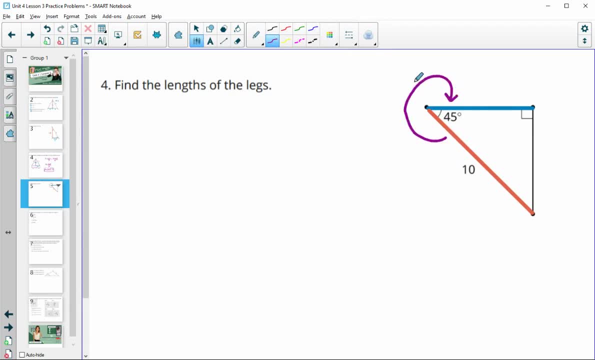 So if you have the hypotenuse, that's the longer one. So when you go back to the leg, you want to divide by the square root of 2.. So this blue segment here is going to be equal to 10 divided by the square root of 2.. You can write it like this as well: 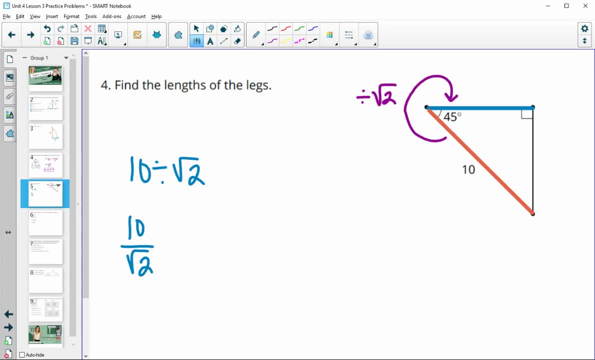 And you could simplify the radical here, which would mean that we would want to rationalize and not have a square root in the bottom. So we'll multiply both top and bottom by the square root of 2. And that gets us 10 times the square root of 2 on the top, And then the 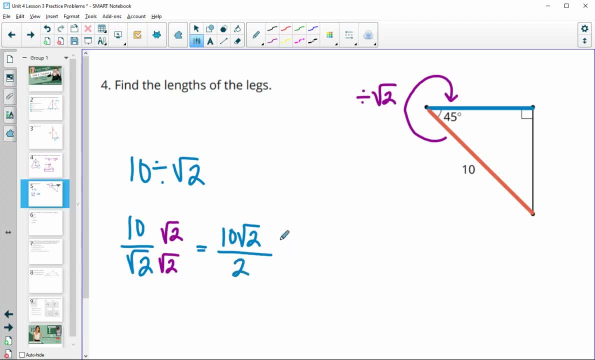 square root of 4 on the bottom, and the square root of 4 is just 2.. And then we could simplify here: 10 divided by 2 is 5.. So we would end up with 5 square root 2.. So one of the answers. 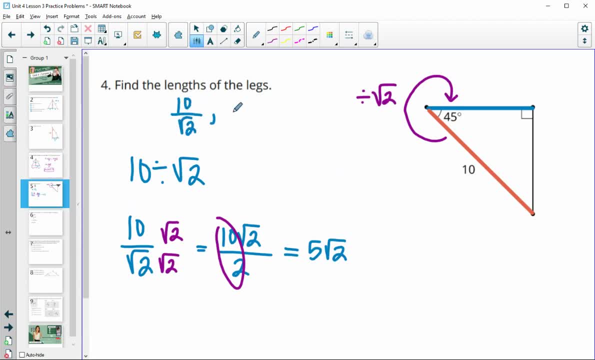 so maybe you're allowed to leave it as 10 over square root 2.. That's fine. Another way to write it is 5 square root 2.. And then the other way to write it would be to do the decimal. So actually. 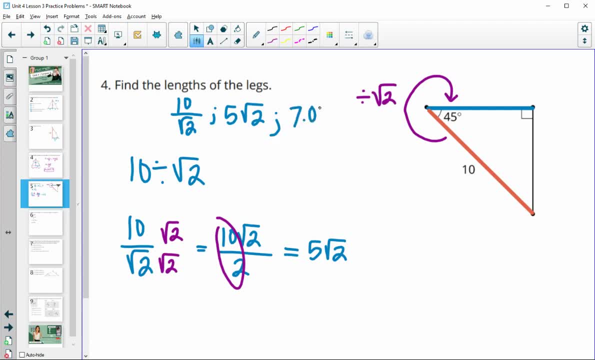 multiply 5 times the square root of 2.. And then we would end up with 5 square root 2.. So that's a 2. And you would get 7.07.. So kind of any of those answers are fine. 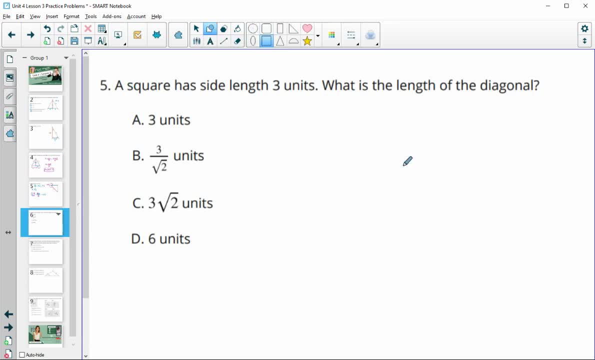 Number 5, a square has a side length of 3 units. What is the length of the diagonal? Okay, so we're looking for this And remember that the relationship between the diagonal and the side is that they're a square root of 2 factor different And the hypotenuse is longer. 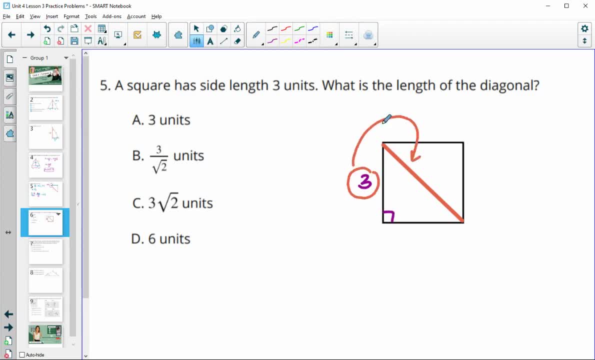 Okay, so you're going to take the diagonal and the side and you're going to take the diagonal and you're going to take this one and you're going to multiply by the square root of 2 to get the hypotenuse. So this is going to be 3 square root 2.. And so we can look and we can see. 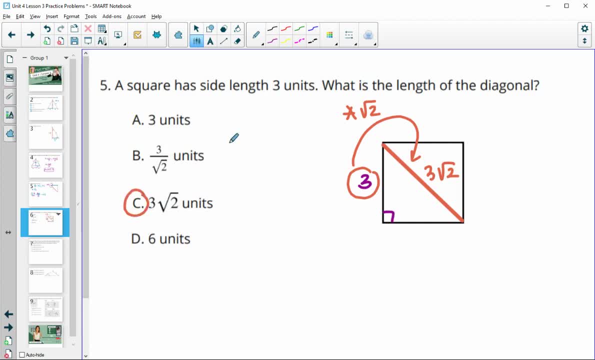 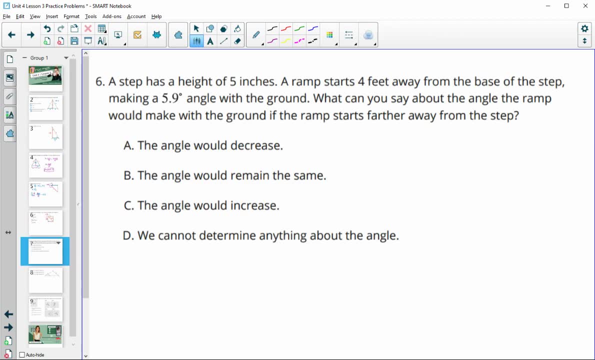 that 3 square root 2 is one of our answers And it just wants us to select one answer, So C is the correct answer. Number 6, a step has a height of 5 inches and a ramp starts 4 feet away, So let's. 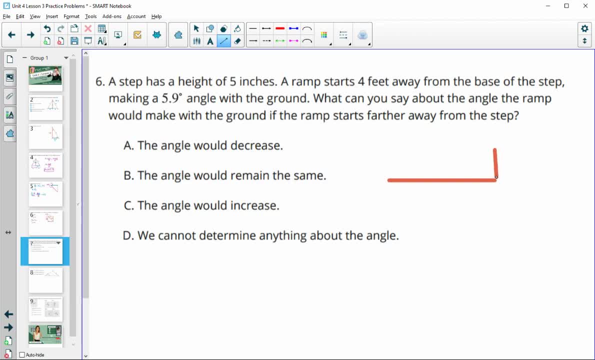 draw this out. So we have a ramp starting 4 feet away from this step And the step is 5 inches, And this ramp is 4 feet away from the base, making a 5.9 degree angle with the ground. So this angle in here is: 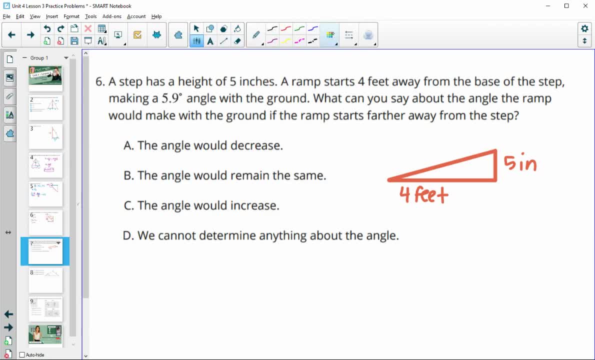 5 point, oops, is 5.9 degrees. What can you say about the angle the ramp would make with the ground if the ramp starts further away from the step? Okay, so if we were to take this and move it further away? so extend, let me. 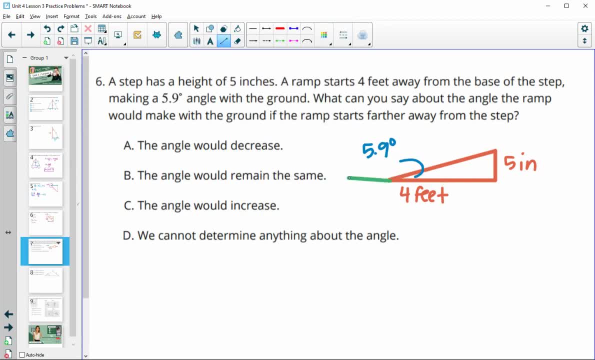 get maybe a different color here. So if we were to extend this further, what's going to happen to this angle here? So that angle is going to get shorter. if the step stays the same height And we just keep pulling the ramp further and further away, then the angle would decrease in size. 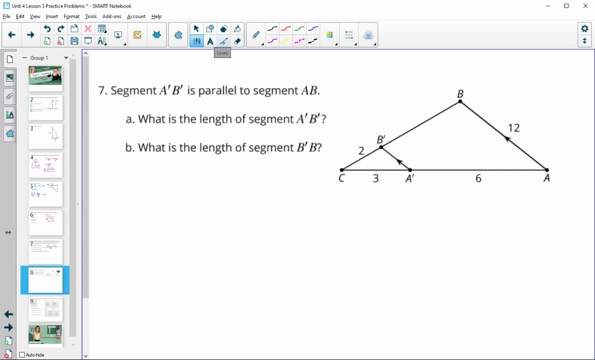 Number 7, segment A prime B prime is parallel to segment AB. So this one is parallel to this one. What is the length of A prime B prime? So this is the base of kind of this triangle here. And then the other segment is the length of A prime B prime. So this is the base of kind of this triangle here. 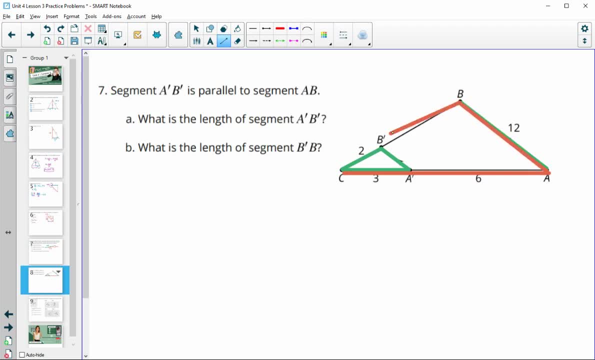 So this is the base of this larger triangle. So we'd want to find the scale factor that connects those. So we've got, if we think of AC as the original segment, okay, and A prime, C as the new. so we would do the new divided by the original. Okay. so three: the green segment divided by the. 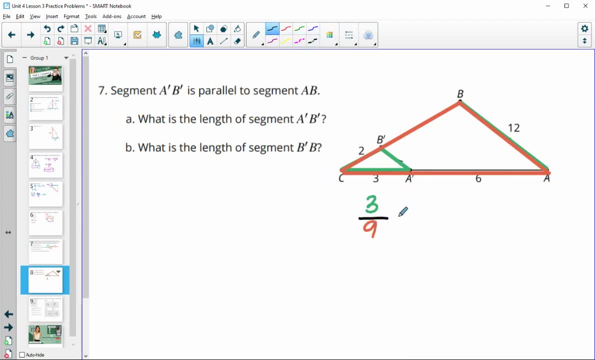 original orange segment, which was nine. So we can see then that our scale factor is one third, So this green segment is going to be one third the length of its corresponding part, 12.. So A prime, B prime, is going to equal one third of 12, or 12 divided by three, So that is going to be four. 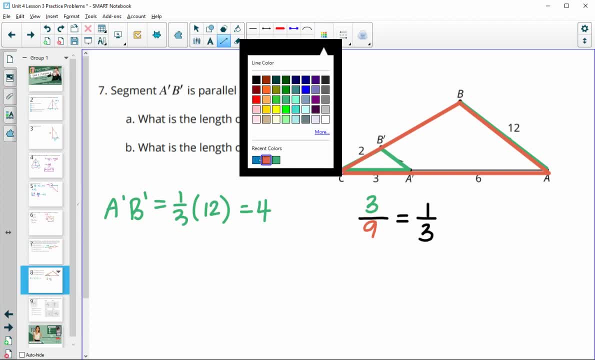 Then it wants to know the length of BB prime. And now this is just a chunk of the side. Okay, and we know that these little, these segments here are proportional. So we can just look at how the three is connected to this six. So to get from three to six we would multiply by two. So then we're going to do the 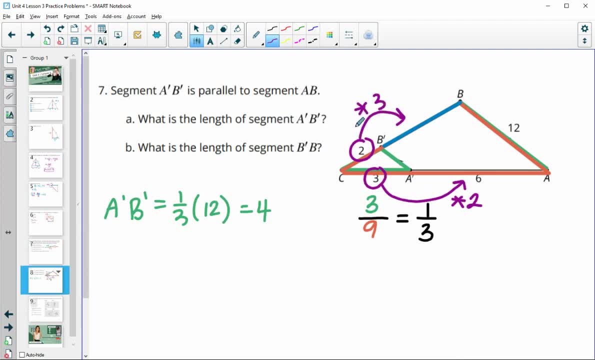 same thing here, two times three, Okay, Or sorry times two. So multiply the three times the two to get the six of this two. we're going to multiply by the same amount, So multiply that by two and we get four. So B prime, B is going to equal. 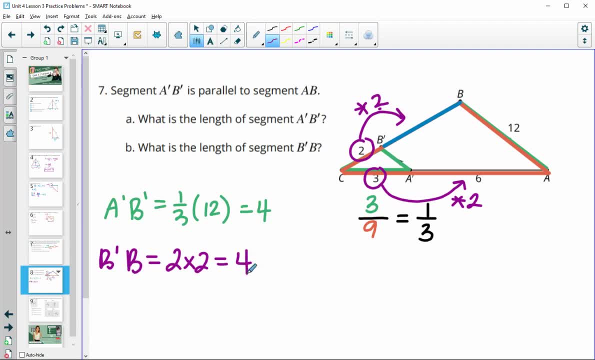 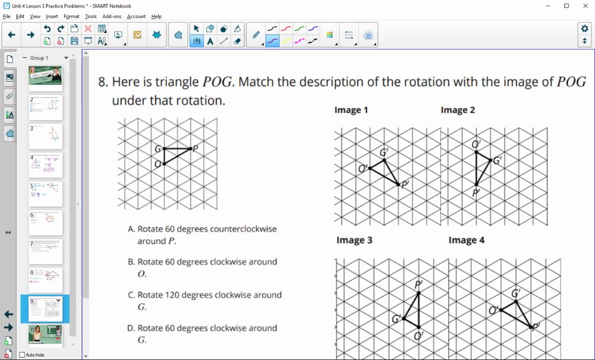 to two, two times two, which is four. All right. and then this final problem here is saying that we've got this triangle POG match the description of the rotations, okay, under each of these rotations. So one thing I like to do in: 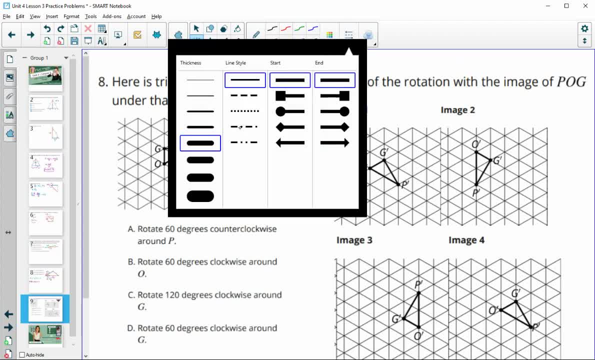 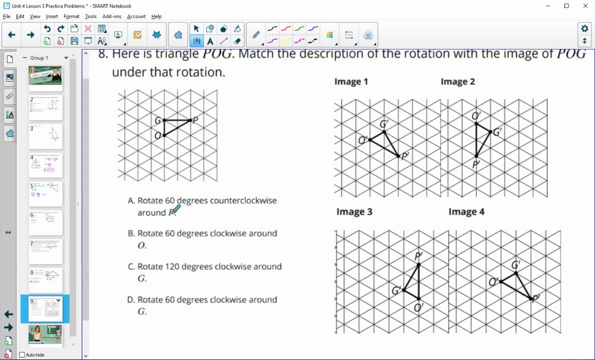 these is decide which point stays the same in each option, because that's going to be your center of rotation. And in A, P stays the same, in B, O does, and then in C and D, G does. So if we can figure out which, 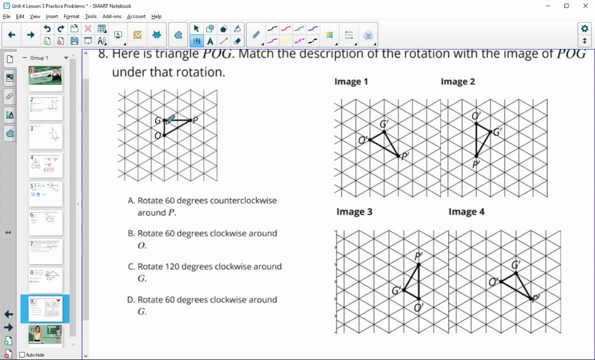 drawings keep P and O in the same. we already know them, So let's take a look here. So image one: this point G is staying in the same spot. And also in image two, G stayed in the same spot. Image three: it has P in this same spot. Okay, so P, prime and P are in the same spot. 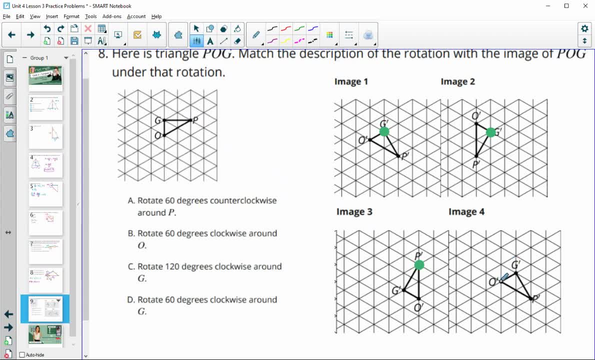 And then in this one O stays in the same spot, So we can kind of see that in the same space there. So then this helps us to narrow down our options. So the one where P stayed in the same spot is image three. So this is the 60 degree clockwise rotation In image four. O stayed in the same spot. 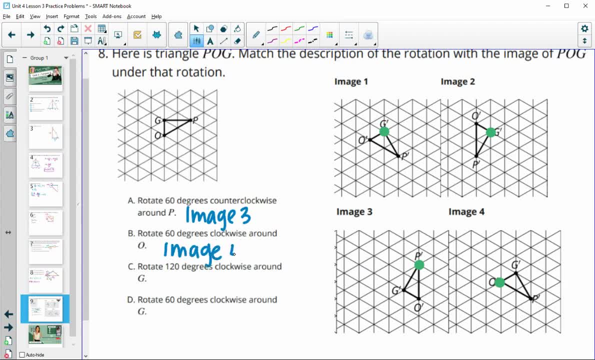 So this is the 60 degree clockwise rotation around O. So now we just need to look at these two and decide which one is a clockwise rotation- 120 degrees. So let's take a look here. If we did a 120 degree clockwise rotation, so remember, clockwise is this way. Okay, so this segment. 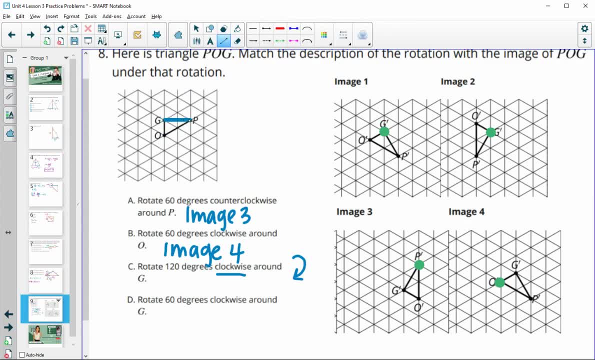 here and maybe I'll erase some of this. This segment here is going to rotate, kind of two triangles worth. I don't like this because it splits one of the triangles in half, So I'm going to look at this one. Okay, and this one needs to.